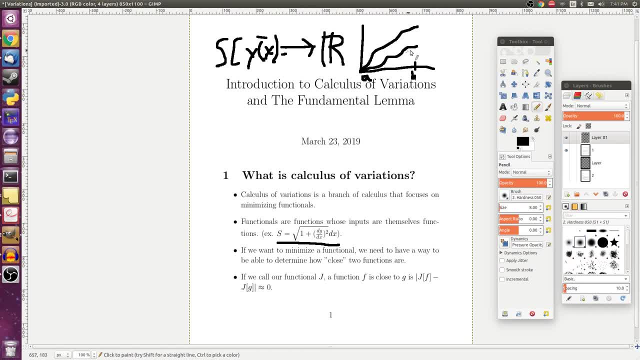 And each of these curves would have a number associated with them, This number being the length of the line. So sometimes, well a lot of times, especially in physics, we're going to want to minimize or maximize these functions- functionals. But for that term to make any sense, we need to be able to determine how close. two. 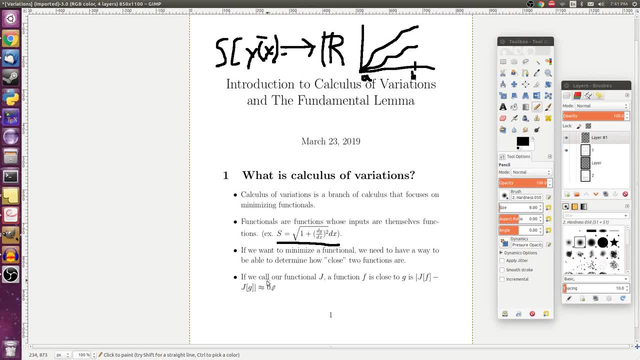 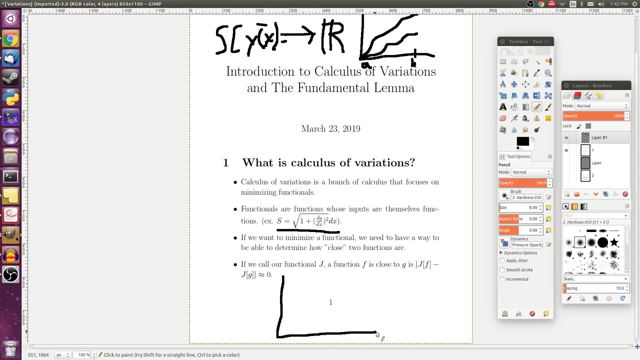 functions are. So for a functional j, two functions, f and g, would be close to each other if their difference after applying that functional would be close to zero. So just to make that a little bit more concrete, if we took two curves, like maybe this one and then one that kind of straddled, 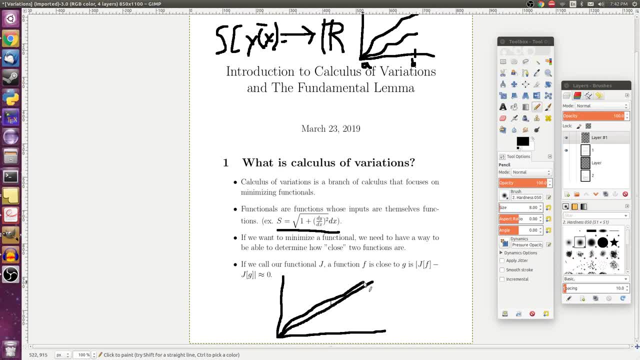 along that curve and we use this arc length functional from earlier. So let's say this length right here is one, And maybe this length right here is one point. Now we could also choose another function that would be pretty close to it by just having 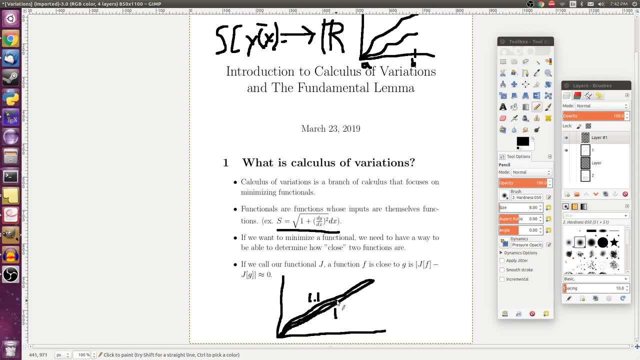 one that's even closer to this curve. but the idea is that if you want to find how close two functions are, you just apply that functional. So for each of these lines you would compute their arc-linked integral and then compare that number that got spit out, because any functional is going to output a real number. 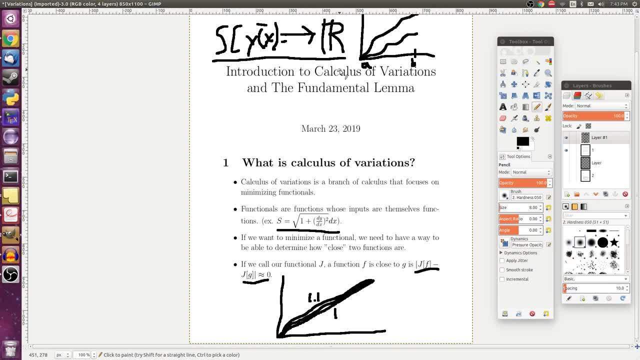 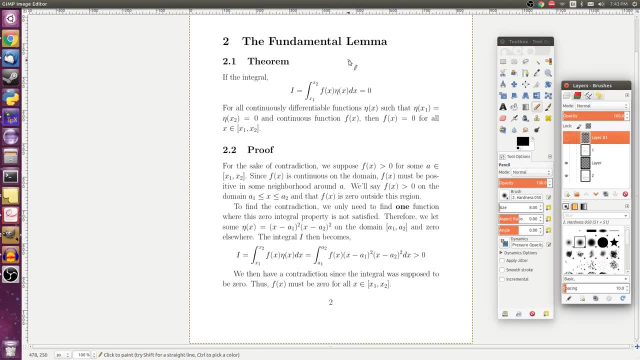 so you can always determine if they're close- two functions are close- by looking at the output of their functionals. So now we're going to talk about probably the most important limit. So the first thing we're going to do is we're going to do a little bit of proof and 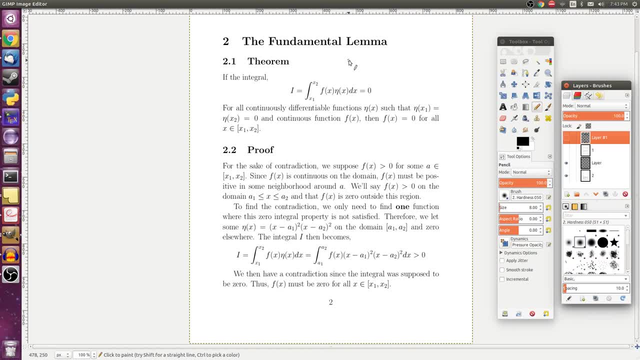 we're going to do a little bit of data or proof in the calculus of variations, because it's going to help us prove a lot of things. So, although this seems like it comes out of the blue in the next video, we'll actually 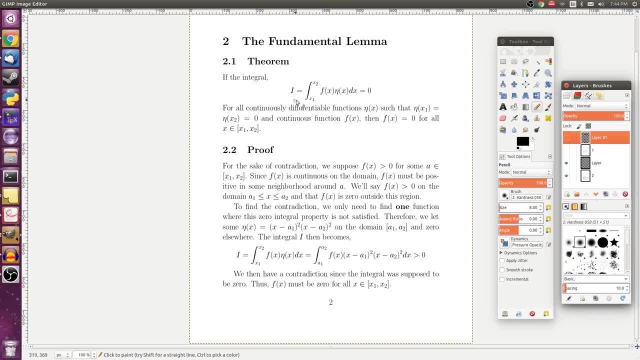 run into our first application of this theorem. So the theorem states that if some integral i from x1 to x2, of f of x times eta of x, dx is equal to zero For any continuously differentiable function, eta, such that eta of x1 and eta of x2 is zero. 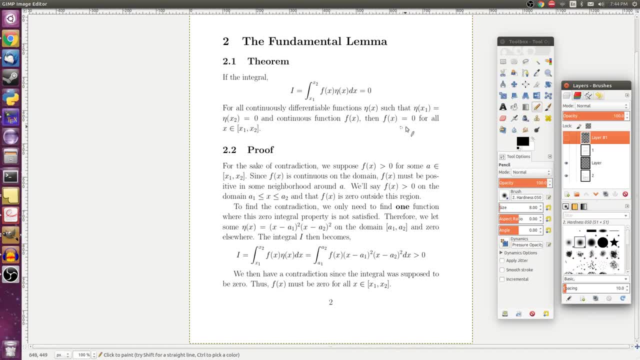 and continuous function f of x, then f of x has to be zero for all x in that region. So if we wanted to draw this out, then what we would be saying is that if you were taking some integral between two points, Two points- x1 and x2, then if this integral is zero for any eta of x, so that it that 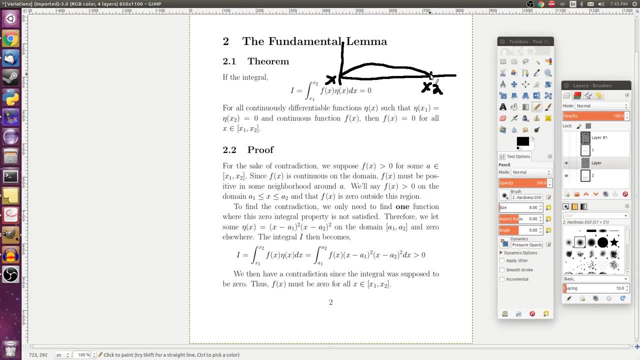 eta of x is zero between these two endpoints. for this integral to be zero, then f of x had to be zero at all these points. Now you may say, oh, that's pretty obvious, But we need to actually prove it. 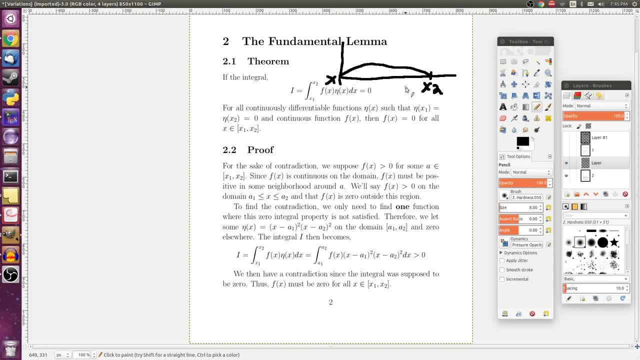 You can't just take something for granted because it seems obvious. So for this proof we're going to use contradiction. So if you want to prove something by contradiction, you get the first part to negate the second part. So if you negate the second part, you get. 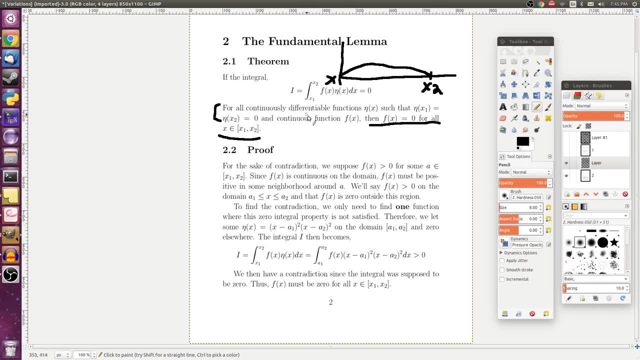 You would suppose Instead that f of x is not zero. So it doesn't matter if we say it's positive or negative, So we'll just say it's positive, just because we have to choose something. So we'll say that f of x is greater than zero for some point a in that domain. 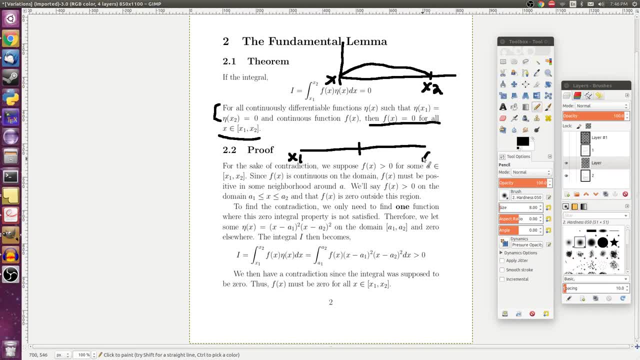 So let's say we've got x1 right here, x2 right here And we've got our point a right here. And then, since we're doing proof by contradiction, we get this first part for free. So we get to assume that eta of x is some function that disappears at the endpoints. 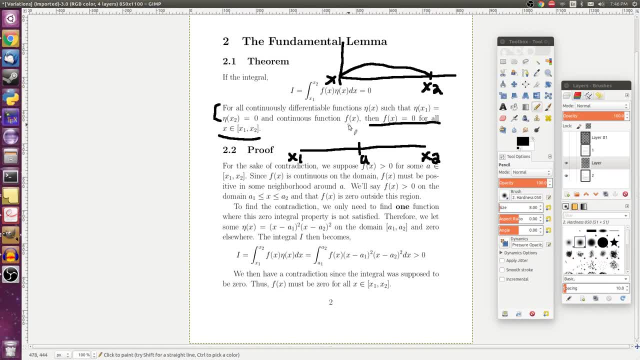 and that f of x is continuous. Now the second part- f of x is continuous- is going to be very important because since f of x is continuous, Then if it's positive at a, then it's going to have to be positive in some neighborhood. 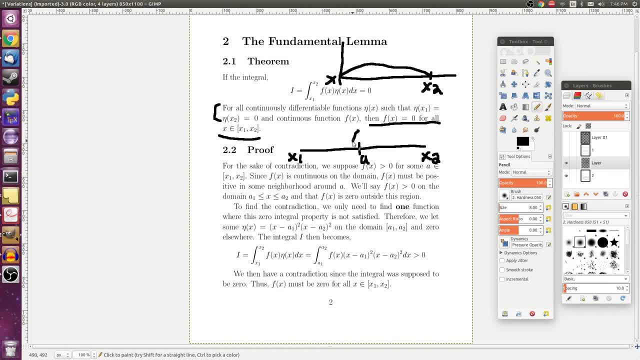 around a. So in other words, it would have to be something like this: And then we'll say that f of x is zero outside this region because we only really get to assume that it's positive at a. And then we'll say that f of x is zero outside this region because we only really get to 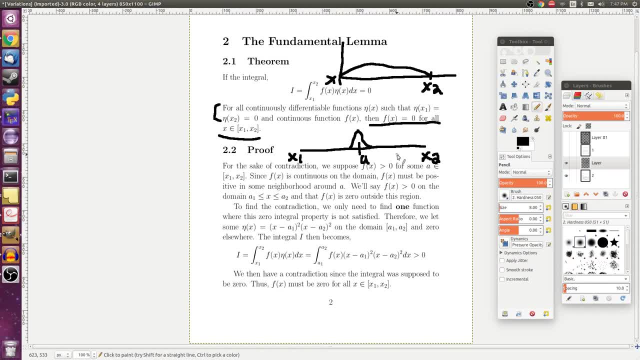 assume that it's positive at one point. So by it being continuous, we know it would have to be continuous in some region around that point. Positive I mean. Then we'll label this region as a1 and a2.. So to find the contradiction that we're looking for, we need to find one function- eta- where 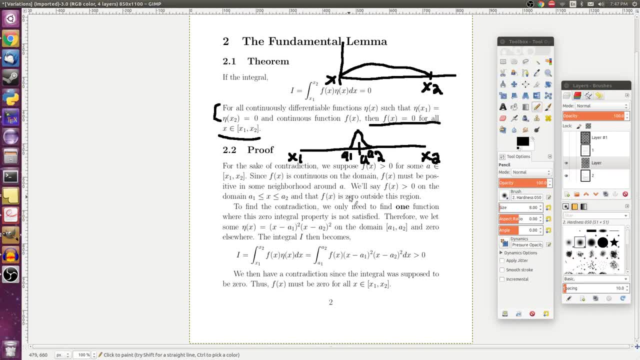 that zero integral property is not satisfied. So if we let eta of x equal to this function right here, So first off it disappears at these endpoints, right here. So it's This: eta is going to be zero here and zero here. 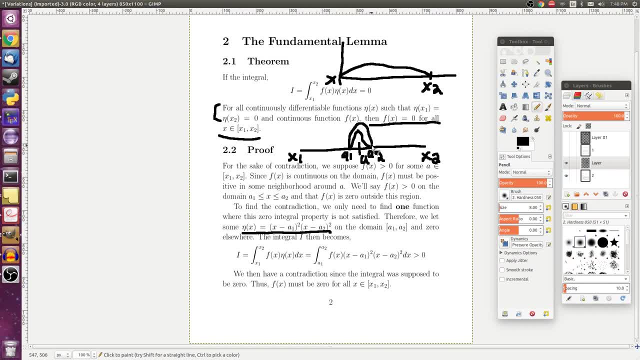 And then we'll suppose it's positive. Okay, We know it's positive because each of these terms is squared. so you're multiplying two positive numbers on that domain And then we'll say that this eta of x is zero outside this region. 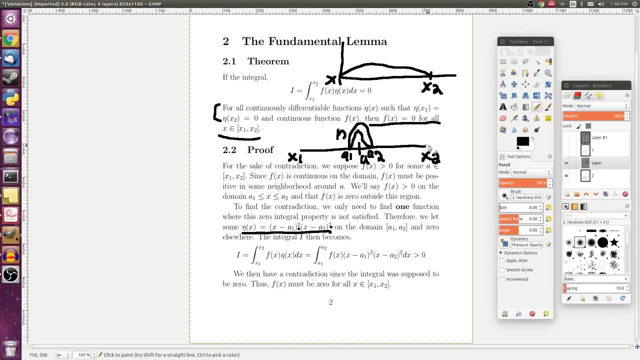 So it's zero from here to here and here to here. So then, that integral from earlier then looks like this: Since f: So So this function on the inside right here was equal to zero and eta is equal to zero in these two regions right here.